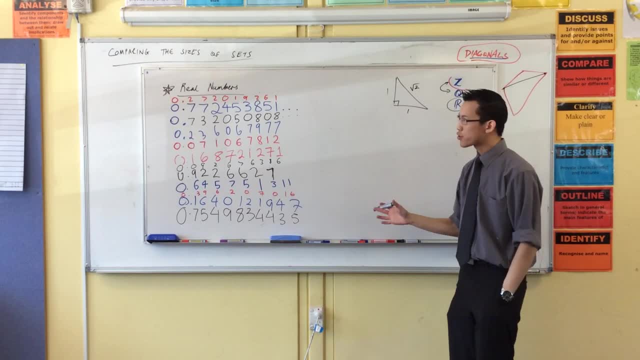 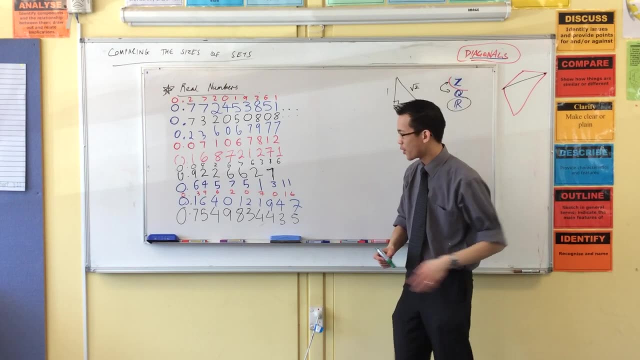 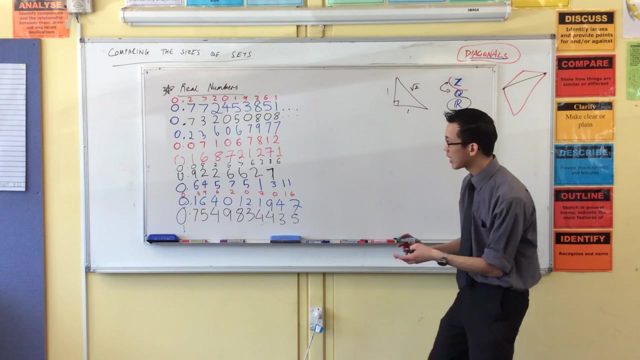 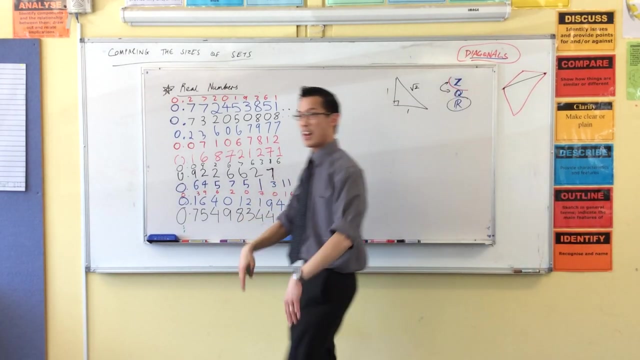 make up numbers as you go, okay, But the point is, what we're trying to do is write down. well, we can't write down all of them, but just imagine that we could. right, So you know, dot, dot, dot, and it just keeps on going forever, right Now? my game before was to say, well, look, okay, here's your real numbers. okay, I'm just going to match these all up to what am I doing? Integers: okay, I can do that, no problems. Look, they all just go down the line like this. so I'll make this match up with one. 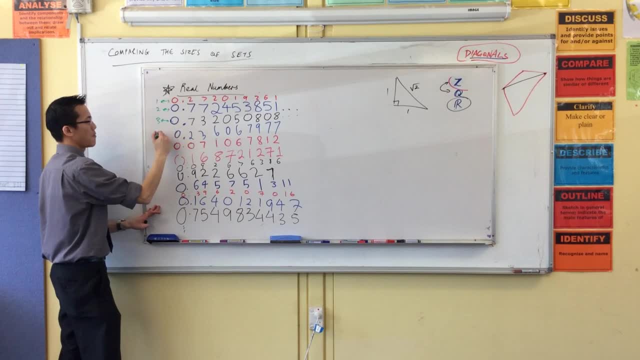 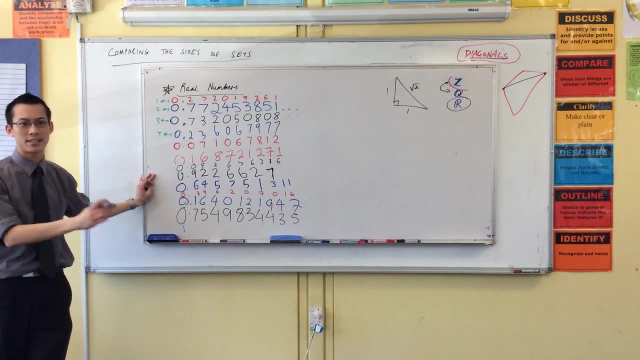 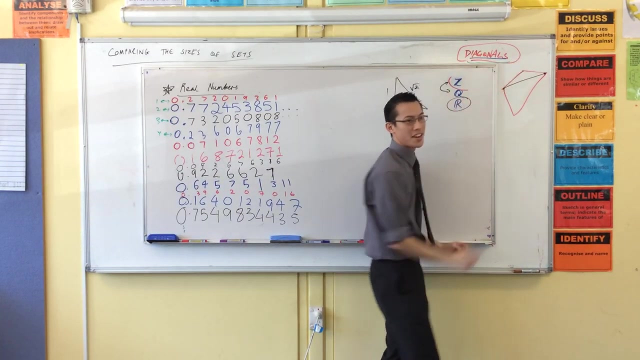 And two and three and four and so on. okay, So you're like, what's the big deal? It looks like I can use the same logic and I can prove that these are the same. Ah, except there's a problem. there's a problem and I'm going to show it to you with another diagonal. Watch this, okay. 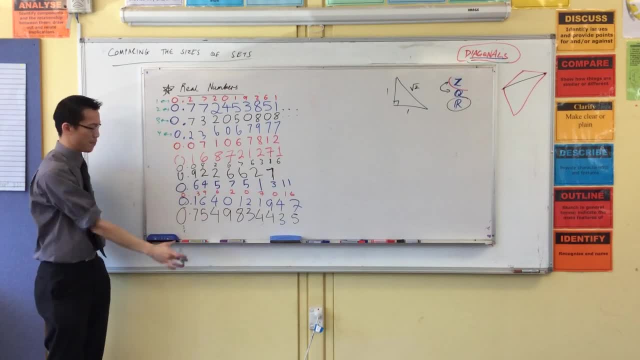 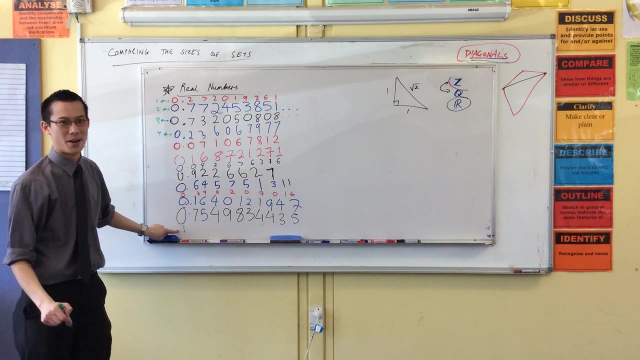 So our assumption was that this list of real numbers, if it went on forever, has all of the real numbers on it. okay, But I'm about to prove to you that no, no matter how long this list goes, this list can go on forever- you'll still be missing a number. Watch this. I need some space. 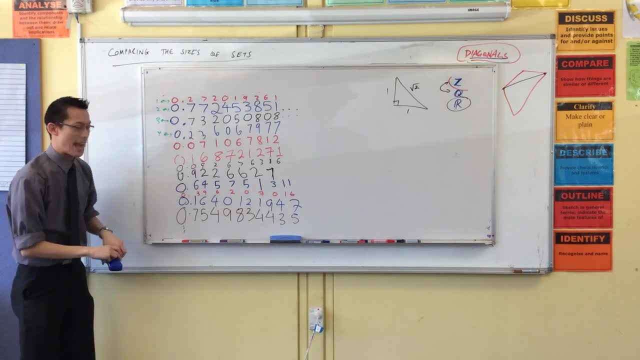 What I'm going to do is I'm going to form a diagonal here, I'm going to make a new real number right, And I'm going to try and show you why. even if this list goes on forever, the real number I make up will be different to every single one that you write down. 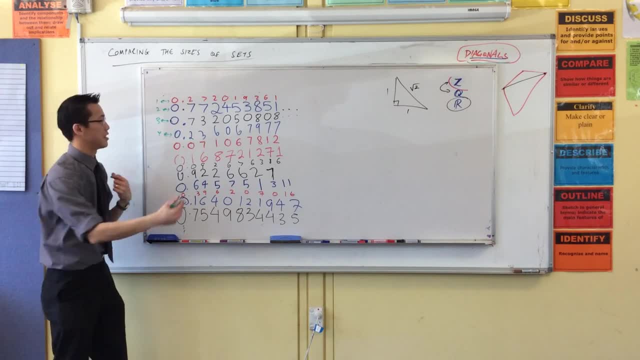 And there can be an infinite number if you write it down. okay, Watch this. I'm just going to start with zero point, because everyone else did so. a bit of peer pressure. okay, What I'm going to do is I'm just going to start with this first number here. 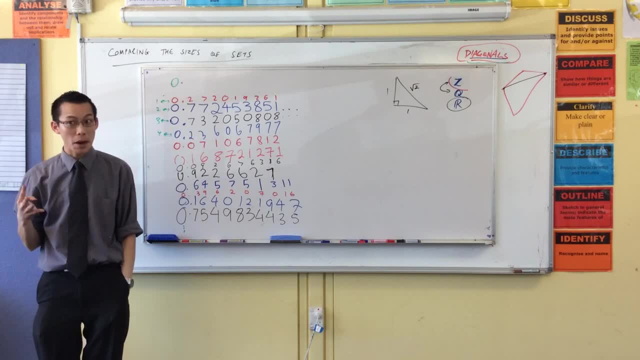 Remember, what am I trying to do? I'm trying to make up a real number that isn't on your list, So I'm just going to say: well, look, if I just look at this first decimal place here, okay, All I'm going to do is in my manufactured number, I'll just make sure my decimal for this first place is different to that one. 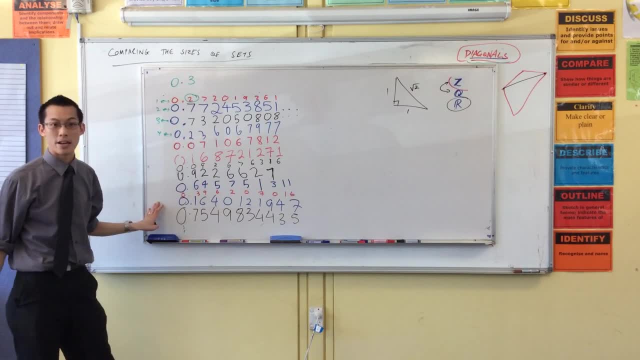 I'm going to make it say: let's just add one, three, okay, Now automatically this: I don't care what the rest of it is. This number is already different to the one that's first on the list. So far, so good. You're like: well, there's a lot more numbers on the list to go. 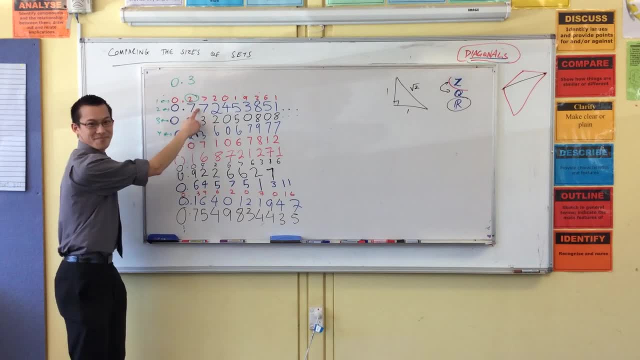 It's all right, I have infinity on my side. I'm going to go to the second number. I look at the next decimal place And I say, well, I don't want to match up with that one either. I'll just make it different, I'll just add one. 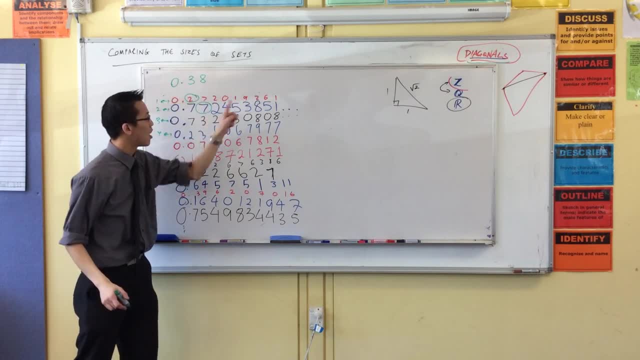 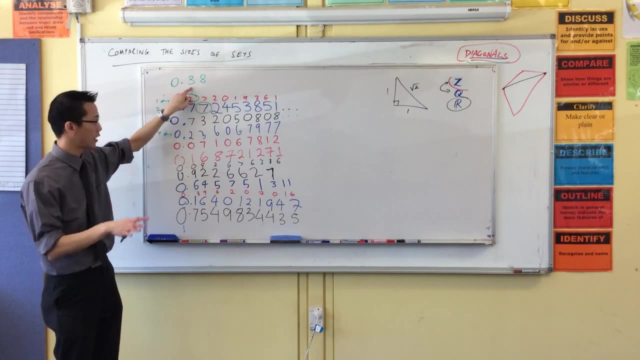 This number, no matter what comes after here or here or here, will always be different than both of these numbers. Does that make sense? Because I've already got this point of difference You're like. well, what about the third number? Well, it's cool. 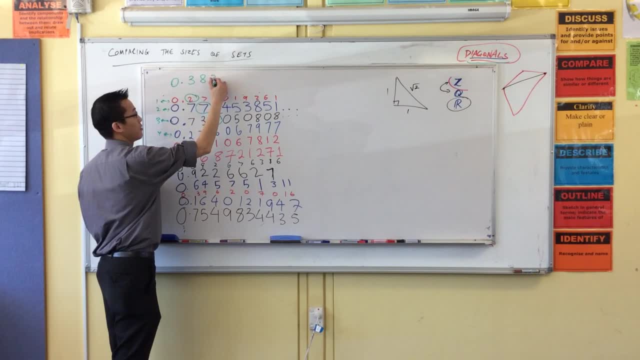 I'll just make sure the third decimal place is also different. I'll just add another one, And I'll make sure it's different to this. I'll add one. I'll make sure it's different to this. I'll add one. 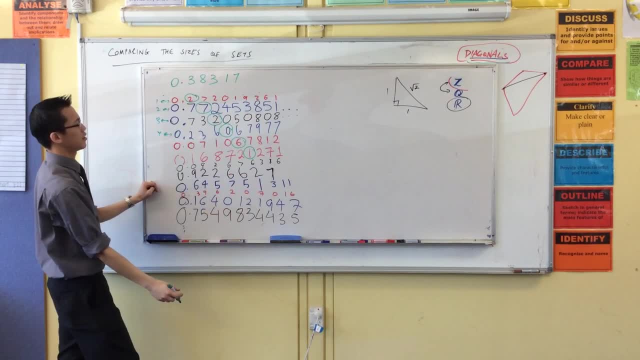 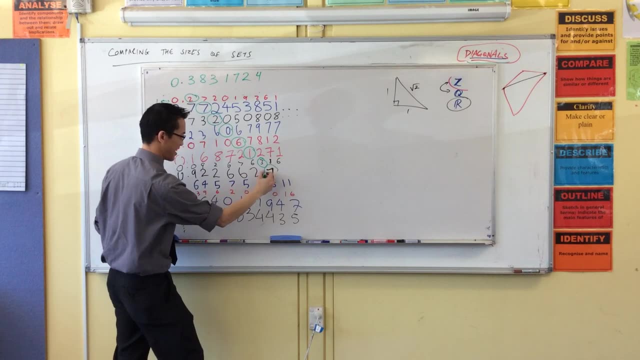 Uh-oh, I'm running out. I think there's one more decimal place on the calculator. Anyway, it doesn't matter, I'll add one. I'll add one. Where does this go? Okay, I think that's that. 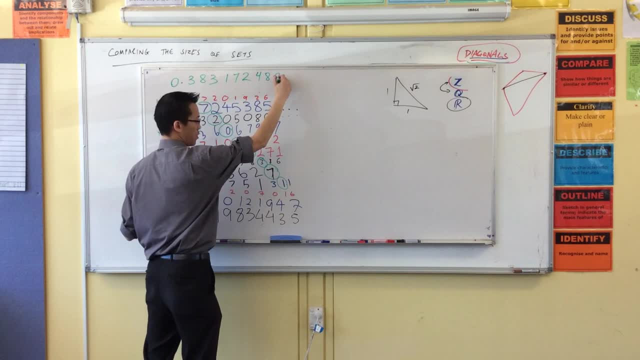 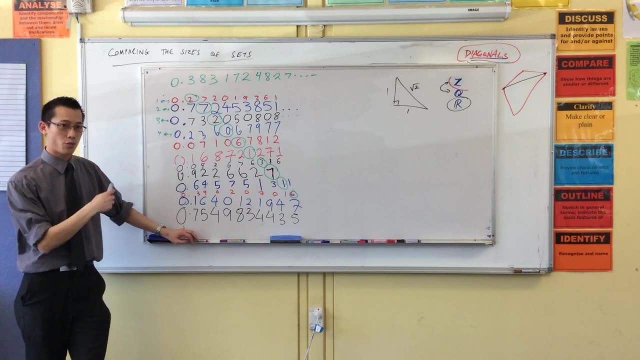 So that's going to be. I'll add one. I'll add one. That's my last one. I'll add one Now. have a look with me: This number that I've just written up at the top in green. This number is clearly different to every number that you have written on the board. 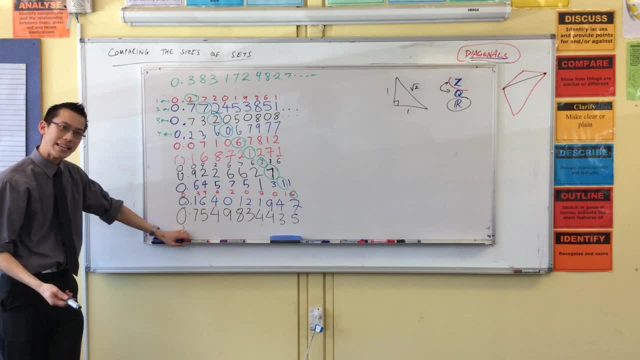 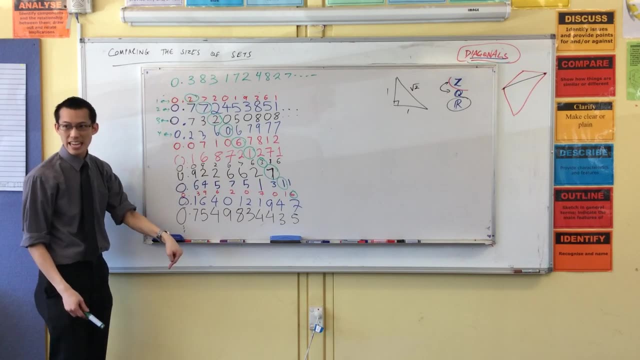 And that's kind of obvious, right, Because there aren't that many numbers on the board. But here's the thing: Your list, which goes on forever. right, My number's going to be different to all of them, Even though your list goes on forever. 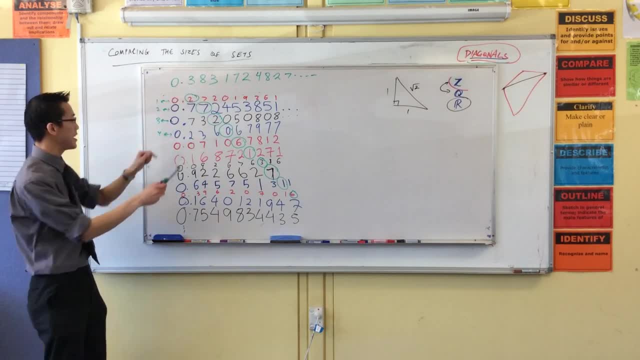 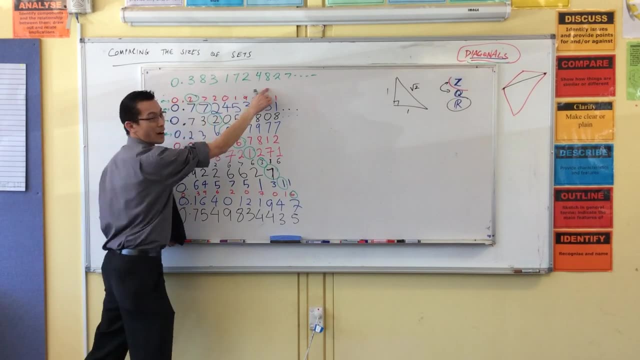 I've got a number that you missed. Remember, this is all about matching up things right. Matching up, matching up, matching up. I found a hole. I found a hole. I can find another hole. Instead of adding one, I can just take away one from every digit, right? 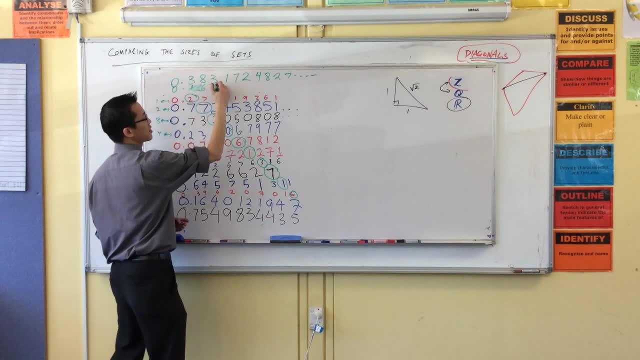 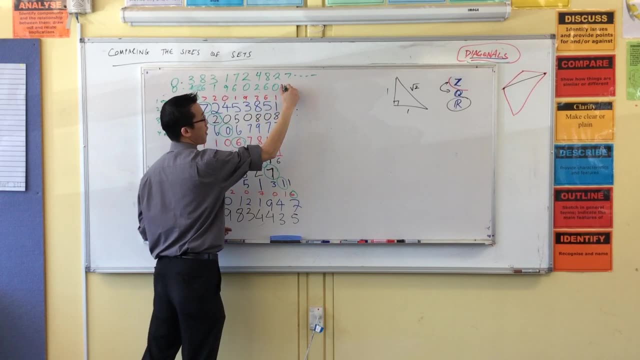 That'll be 2, sorry. 1.. 1, 6, 1, 9.. 6, 0, 2, 6, 0, 5.. Look, this number isn't on your list either, right. 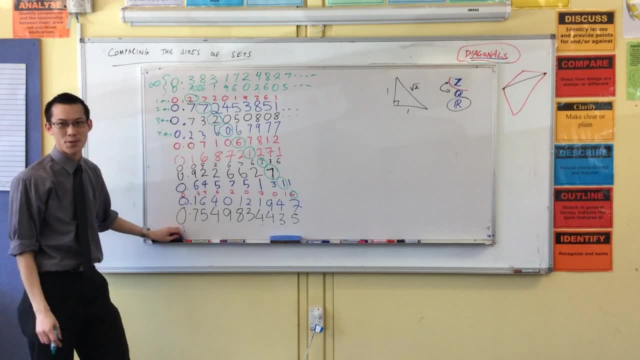 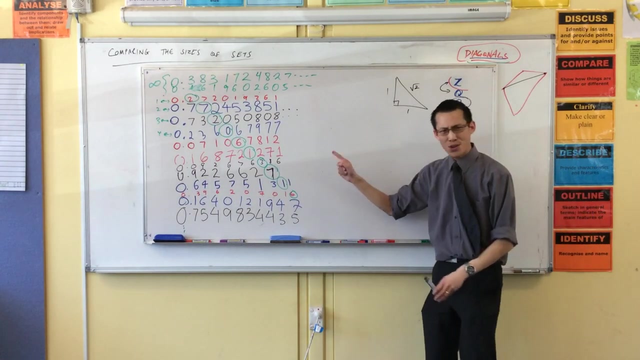 In fact, I can come up with an infinite number of numbers that aren't on your infinite list. It's a lot of holes, okay. So therefore, with a different kind of diagonal, what I've proven is that, even though your list goes forever, right. 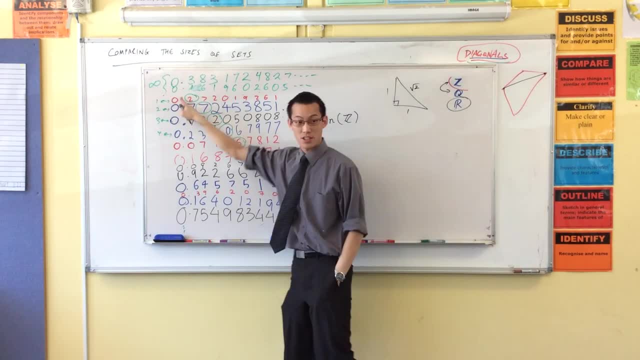 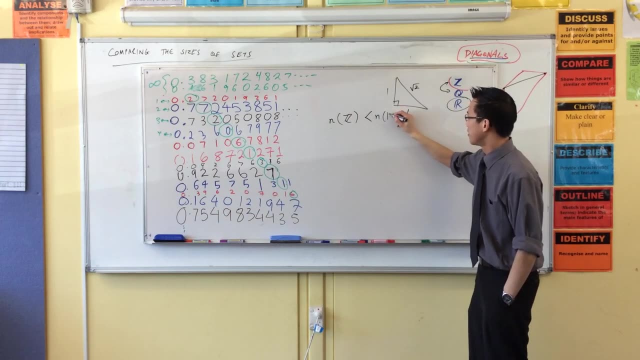 The number of integers, that's how many of these you'll have, because it goes on forever, right, Will always be less than the number of real numbers. okay, Now, this is really mind-bending, right? Because how about all the numbers? 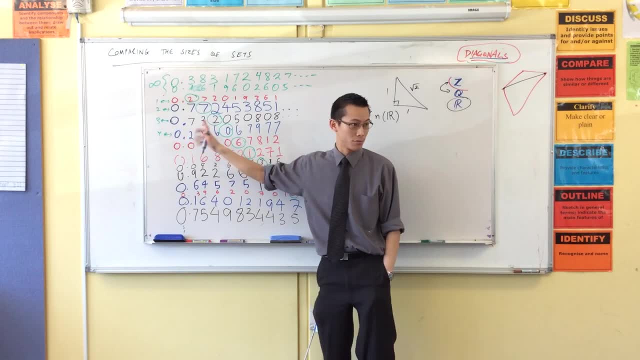 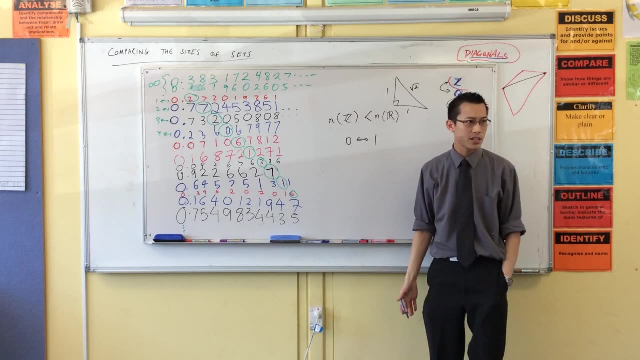 this is why I asked you all to put 0 point on front of your thing, right? All of these numbers. all these numbers are between 0 and 1, aren't they? They're all between 0 and 1? And I've just said that all of these numbers. 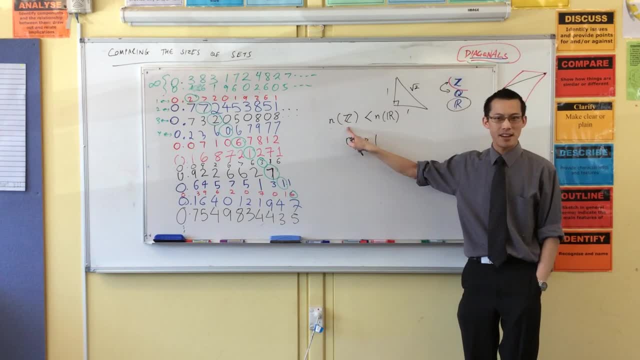 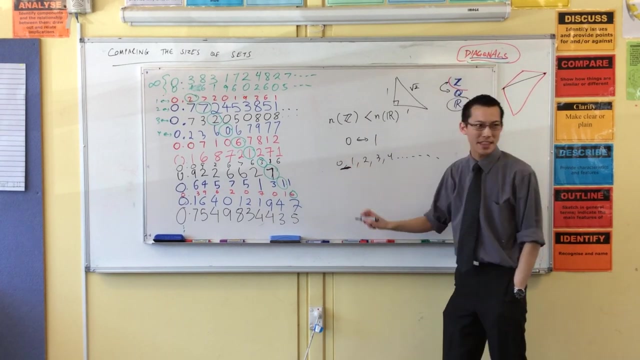 are more than all of the counting numbers, right. So that means there are more numbers between 0 and 1 than there are from 1, 2,, 3,, 4, 5.. Forever. There are more numbers nestled in that little gap there. 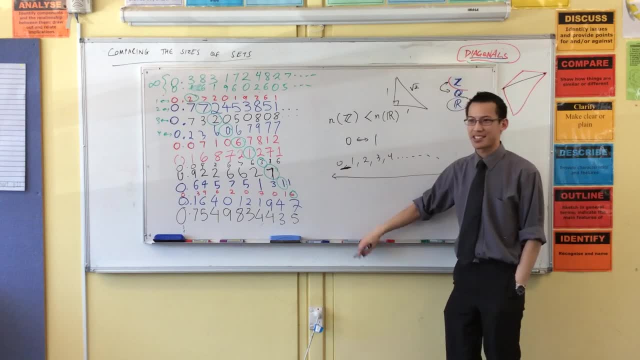 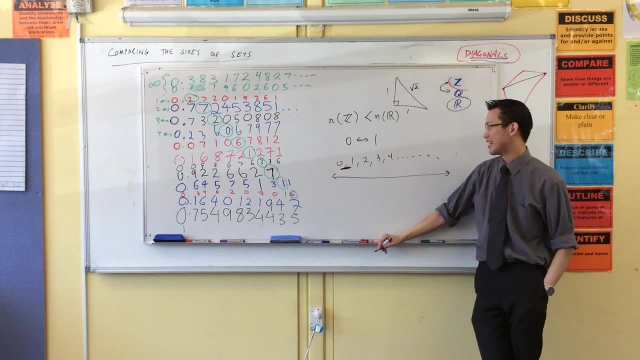 than there are in the whole list. That's weird. That's weird Now to talk about these two different kinds of infinity. it's a bit weird. It's like you know, infinity is less than infinity. That's a bit strange. 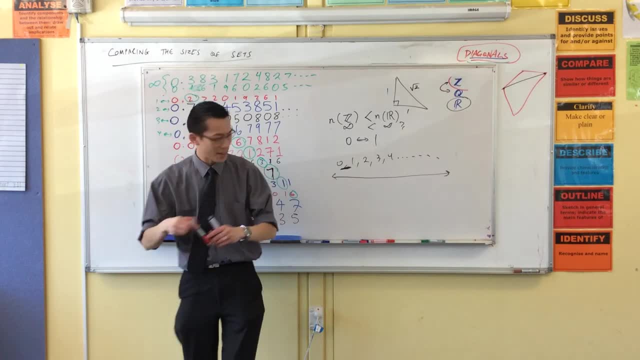 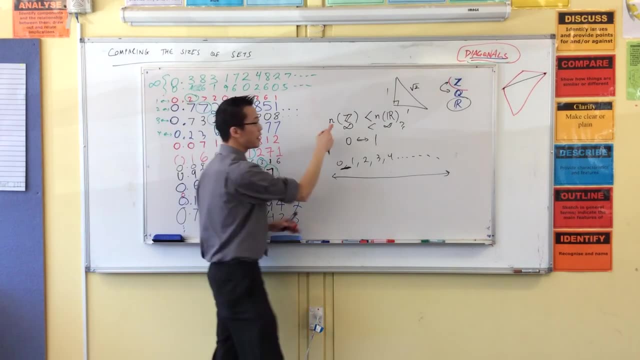 So we need some new language for this, right. Oh, my markers are here. This infinity over here, because it comes from counting 1,, 2,, 3, 4.. We call this a countable infinity, right. 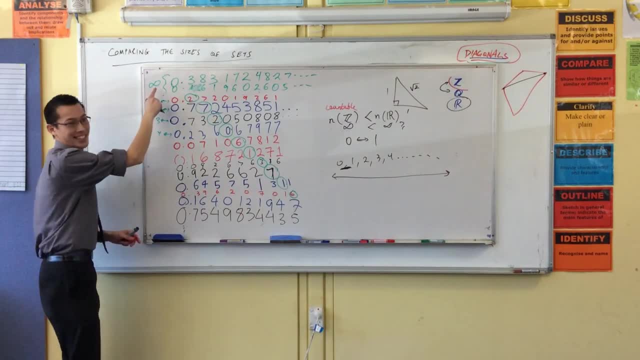 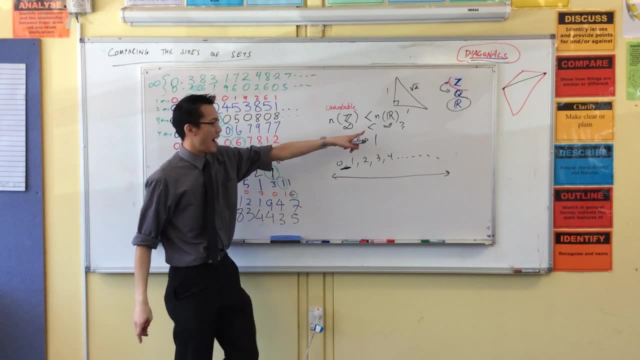 Yes, it's an infinity And it goes forever, but I can count it. I can just go 1,, 2,, 3,, 4, and if I count forever, I'll match up 1 to 1.. This guy, this guy, this is way bigger than this is. 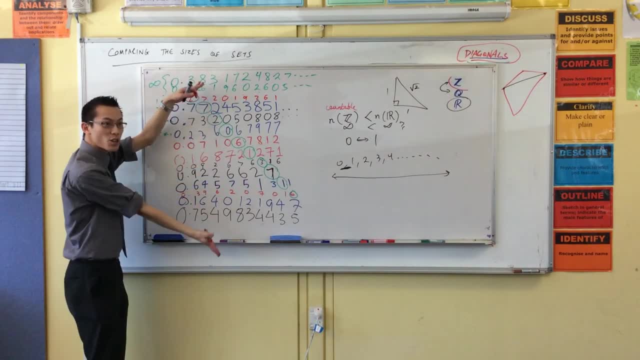 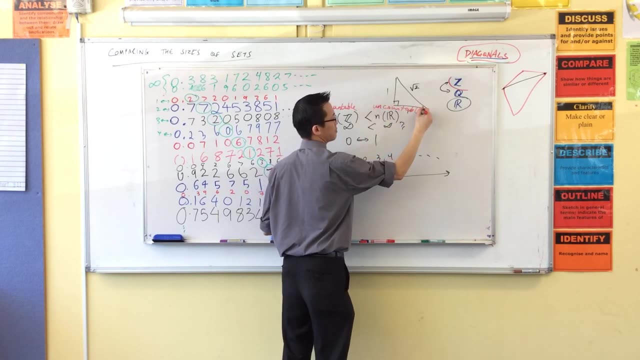 You can't count it. You can't count it. No matter how long you count, I'll always come up with more that aren't on your list. This is called an uncountable infinity. Okay, So you can say: things are sets are countably infinite. 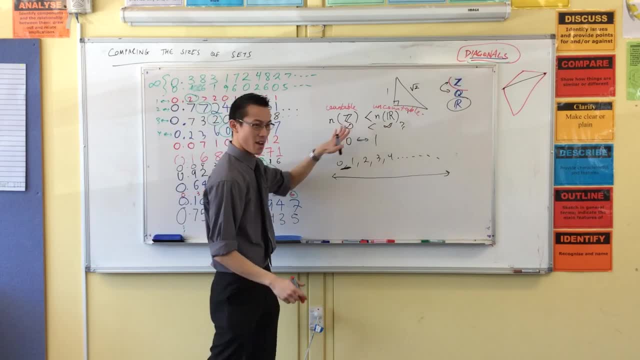 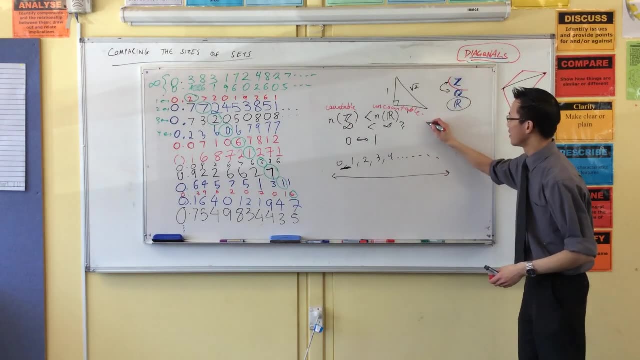 or uncountably infinite, and that tells you how much bigger one is than the other. Now the real question to bend your mind is if you call this like- this is not proper notation, by the way, but you're like: well, okay, countable infinity, right.